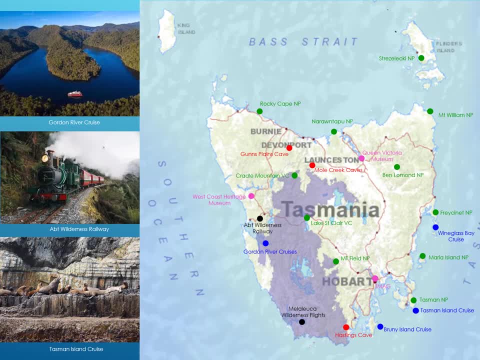 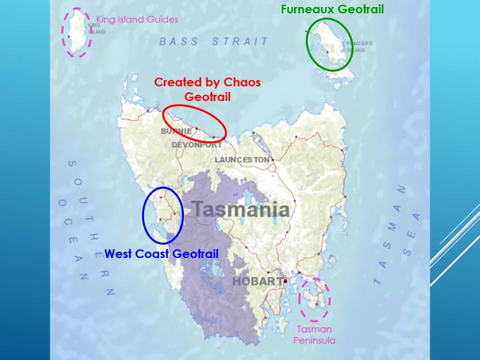 River areas, wilderness flights to Melaleuca and guided cave tours. The wilderness railway provides commentary on the mining history in the Queenstown area. There are first class rock displays at many of the local museums To provide the tourists with greater level of geological interpretation. the tourist 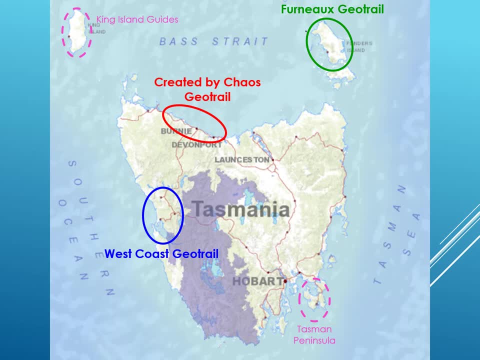 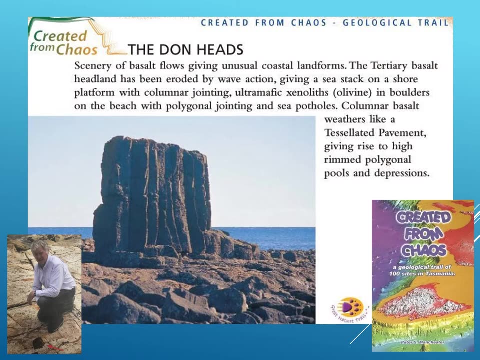 and national park operations are supplemented by three geotrails and local interpretive brochures and signage. The created from chaos geotrail was developed by Peter Manchester, shown in the bottom left, in 2004 to highlight the complex protozoic to paleozoic sequences and cainozoic geology. 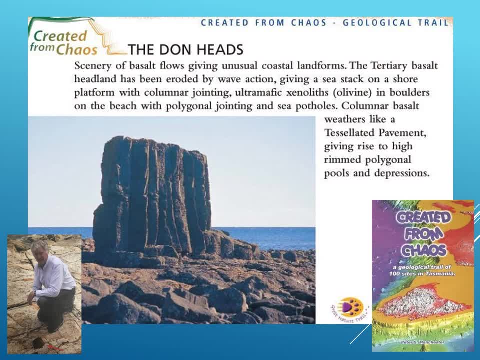 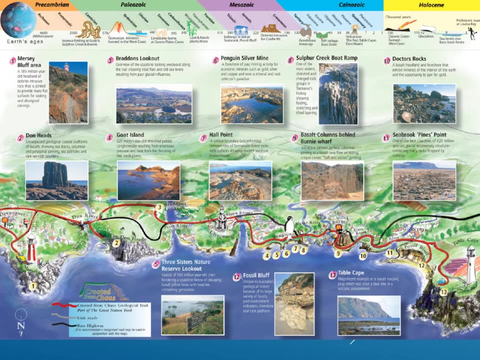 along the north west coast. This concept was later expanded into a now out of print but highly informative book documenting 100 geosites throughout Tasmania. The created from chaos geotrail extends along 60km of scenic shoreline between Devonport's, Mersey Bluff and Wynyards Table Cape and consists of 13 interpretive panels and an information. 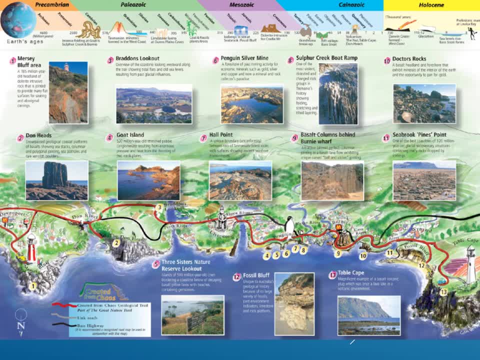 brochure with map. A major upgrade of the geotrail is planned in the next couple of years. The geotrail is now part of the GeoPlanet project. The GeoPlanet project is part of the GeoPlanet project. The GeoPlanet project is part of the GeoPlanet project. 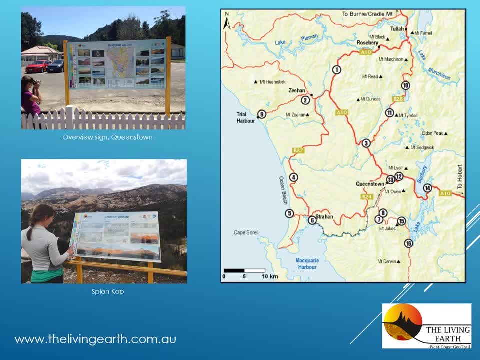 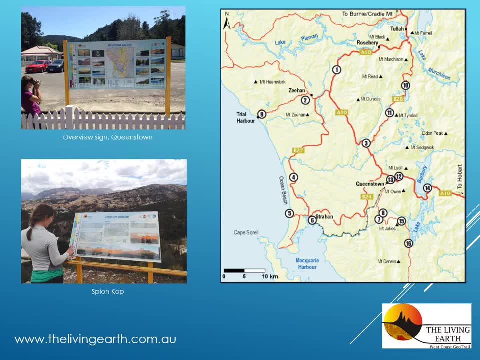 and mining history in the Queenstown to Tulla area in western Tasmania. The geotrail consists of 15 geosites, 6 with interpretation panels shown in the bottom left and 3 overview signs at Queenstown, Zean and Tulla. 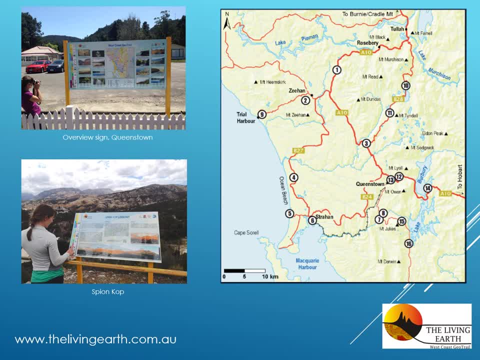 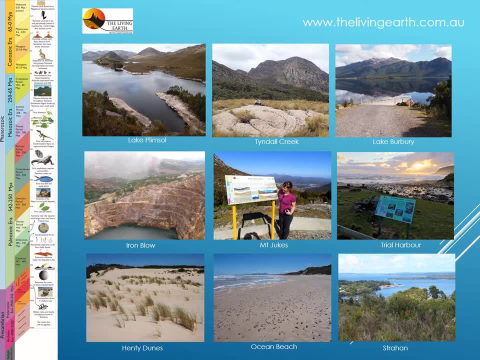 Additional information on the other geosites can be found on the Living Earth website. Extra interpretation panels are also shown on the GeoPlanet site. text to GeoPlanet project are planned in the future. The GeoTrail highlights aspects of the local geology, including the Cambrian to Ordovician rift development. Devonian granite. 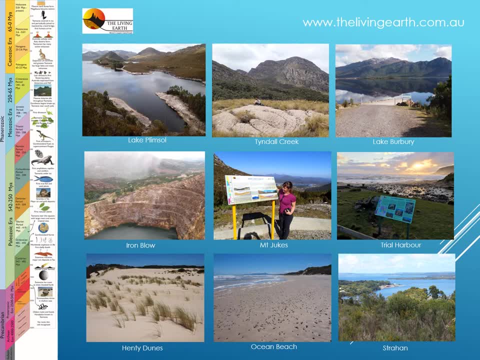 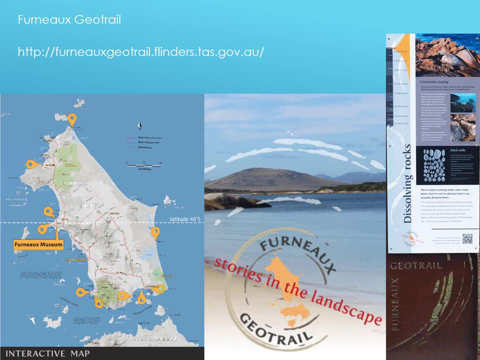 magnetism, mining history and cainozoic landscape development. The Furno GeoTrail highlights the Paleozoic to Cainozoic evolution of the Bass Strait area. Phase one of the project was completed in 2019 and consists of ten interpretation panels, shown on the far right, supported by additional information on the 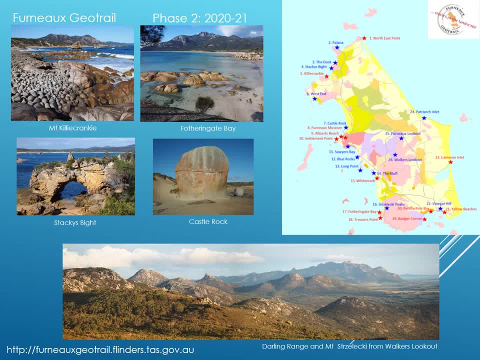 associated website. Phase two of the GeoTrail is currently in development and is due for completion in late 2021.. An additional 14 virtual geosites shown in blue on the map are proposed, with an additional overview sign to be installed at White Mark. 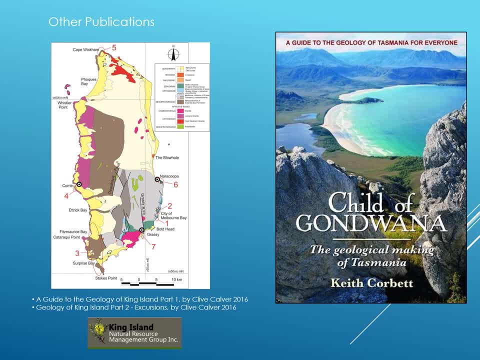 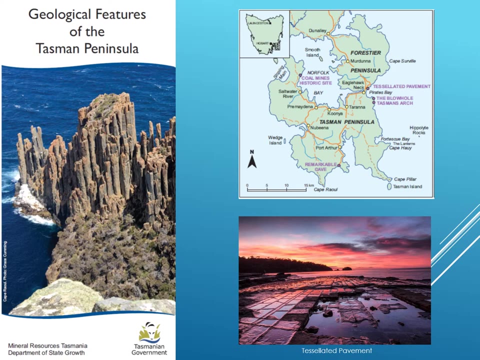 Other notable geotourism projects include the production of an excursion guide to King Island. a non-technical book on the geological evolution of Tasmania and a pamphlet highlighting the geological features of the Tasman Peninsula. A new book describing Tasmanian fossils by 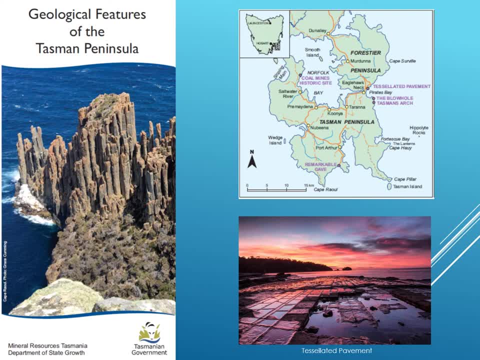 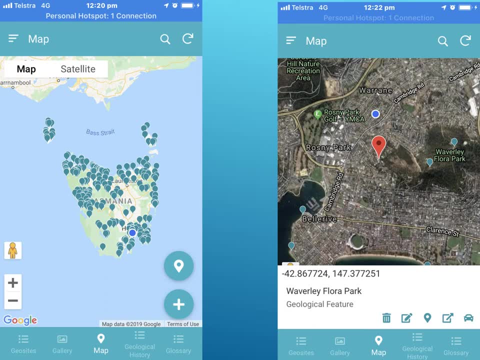 Peter Manchester is due for completion in late 2021.. Future geotourism projects in Tasmania include the publishing of a statewide database of geosites and the development of a statewide geotourism map. The image on the left is from the prototype map showing the distribution. 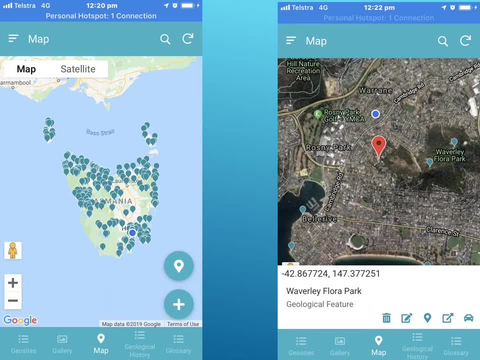 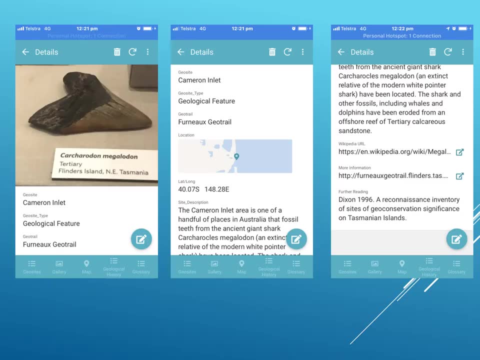 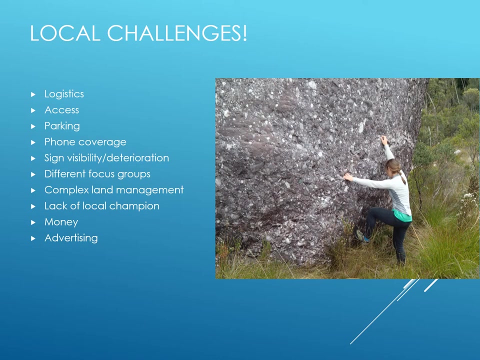 of current geosites in the state. The image on the right is a close-up view showing the selected geosite in Google Earth view. Each site will include a photograph and a general site description with web links for additional information. Despite all best intents, the development of a geotourism project, be it a site-specific, 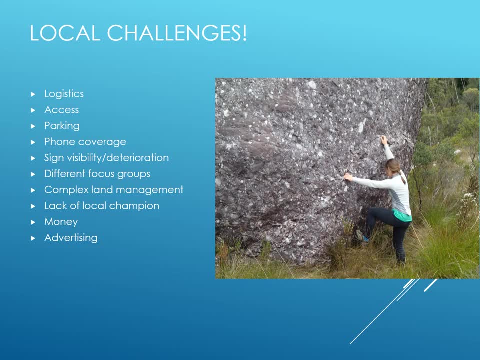 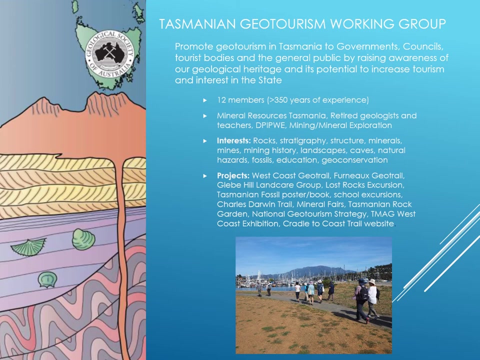 interpretation sign or a full geotrail. the physical, legislative and social landscape of Tasmania provides many challenges which need to be overcome during a project, The Tasmanian Geotourism Working Group was established in 2017.. To address some of these issues and to further promote geotourism in the state,